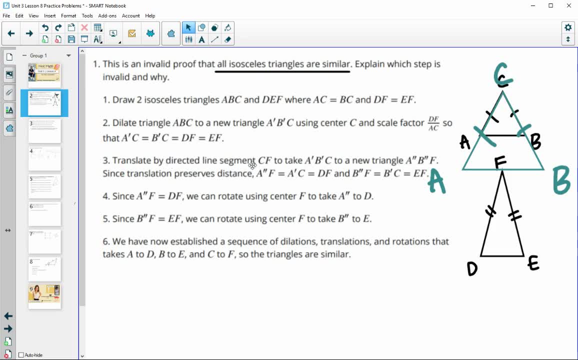 translate this new segment by directed segment CF. so it wants to take us. so we take C to F and it looks like I needed to dilate it just a little bit larger probably, But so translates, let's see. C goes to F, which is going to take our new triangle. take us to another triangle. 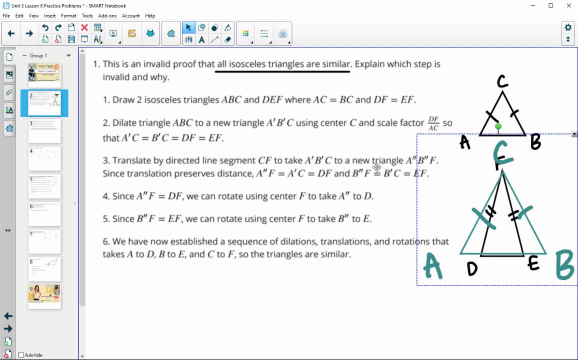 and they just keep re-dilating, Naming them. so just keep looking at my green triangle. But so then that's going to take us to a new triangle. Since a translation preserves distance, we know that A to F is equal to A to C. 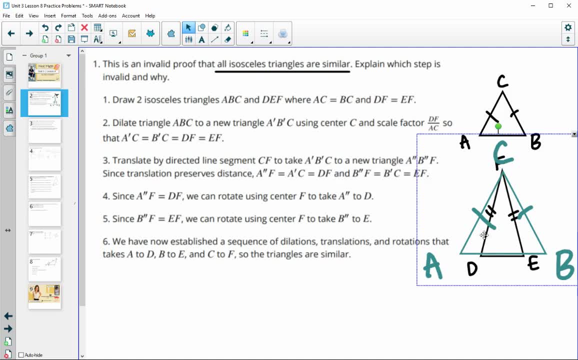 since that's how we dilated it, and also DF, So all three of those are the same, And then B? BF. so if I went from this point to F under here on the black triangle, B, prime, C, prime and then EF. 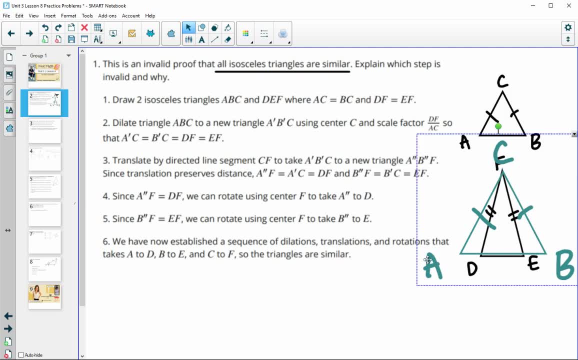 Those are all the same length. so that's fine, You can translate. Then it says now, since we know that A double prime, so again this blue triangle, so ADF, so A to F and D to F are the same length, that we could rotate this until the triangle landed and got those two side lengths on top. 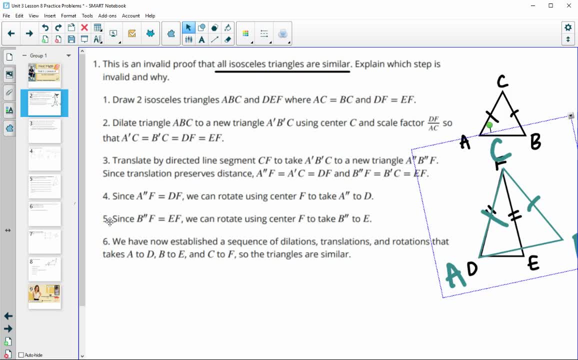 of each other, Completely fine. Then it says: since B, prime, F is the same as EF, so this new green length is the same as this black length. now we could rotate it to put those back on each other. And then it says that we have gotten the entire triangle to be on. 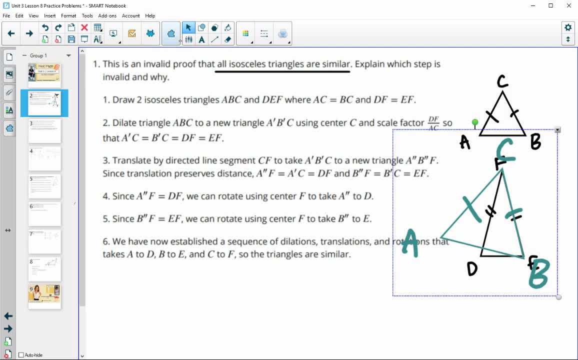 top of the other one. So that's where it goes wrong, because once we rotate a second time- so in this step, when we go to rotate to put B onto E, it moves A off of D. Okay, so rotating A again moves A off of D, and so we don't have a triangle that lands on top of the other one. 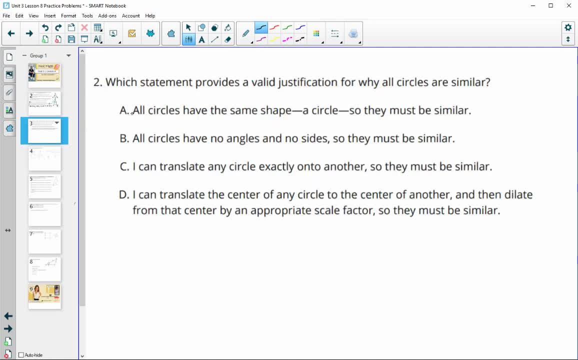 All right. number two, which statement proves a valid justification for why all triangles are, or, sorry, why all circles are similar. Okay, so why are all circles similar? So A says all circles have the same shape- a circle- so they must be similar. I mean. 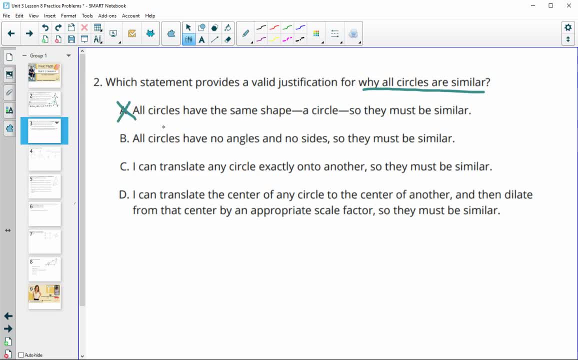 it's close but not quite. That doesn't use our definition of similar okay, because that's kind of like saying all triangles are the same shape, so then they have to be similar. We need a little bit more substance to that. B says all circles have no angles and no sides, so they must be. 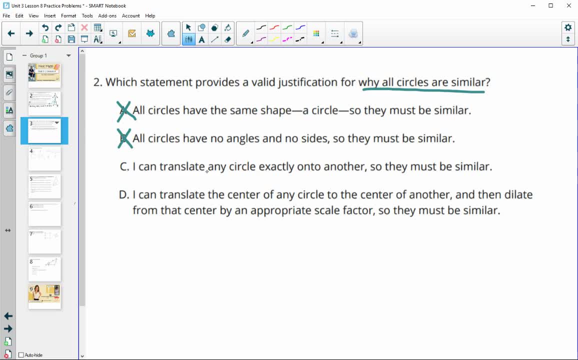 similar. No C, I can translate any circle exactly on the same shape. I can translate any circle onto the other, so they must be similar. That's not true. I mean because if we're going to translate here's one circle, here's another circle, Translating this circle on top of that. 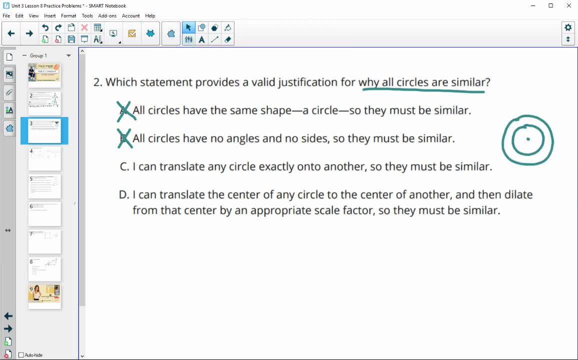 one doesn't land them on top of each other or get them the same side, the same size, so that one's not going to work. I can translate the center of any circle onto the center of another. That's what I did here. Then I can dilate from the center by an appropriate scale factor. 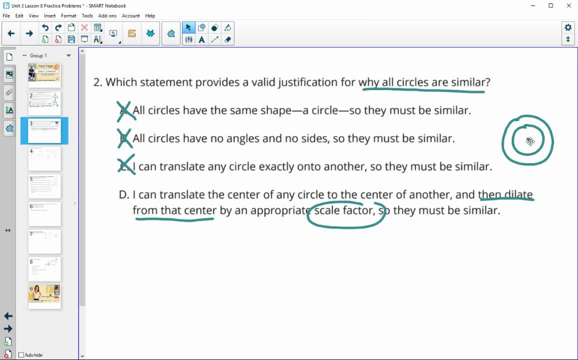 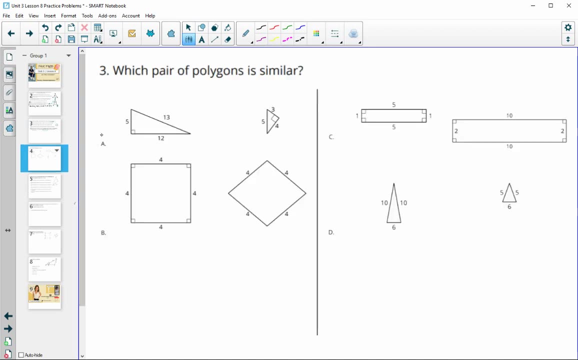 so they must be similar. That would be true because we can take the new radius divided by the current radius and we would be able to get every circle to dilate to the same size. so D, Number three, which pair of polygons are similar? Remember, polygons have to have the same. 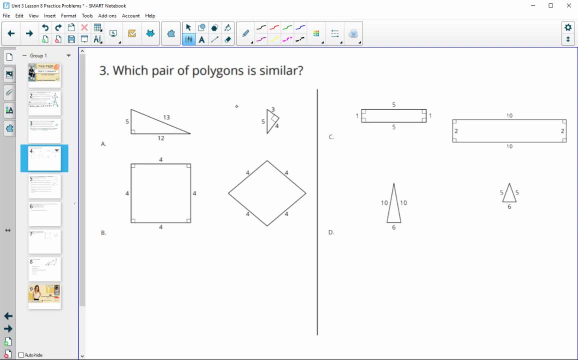 angles and then proportional sides. If we're taking a look here, this second set of shapes we could rule out. This section has no rectangles, but the next set of shapes will make romance- for the second set, That is true- falling down. 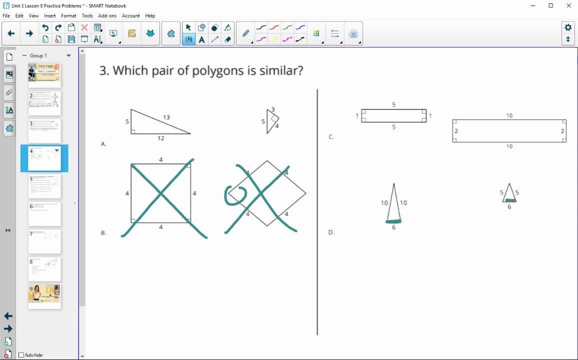 Then we can kind of see they kept this length the same while changing the other side lengths. so these tens divide by two so that sixes stay the same. so this is going to be bad, because they do not have proportional sides. We can look at A and C For A, we can look at the two. shortest sides of A. Once again we've beenHo. it's lower than A, but it's higher than C. Alright, better match. O. oke, Then find the hopper on curves at a higher level Until we accommodate them. 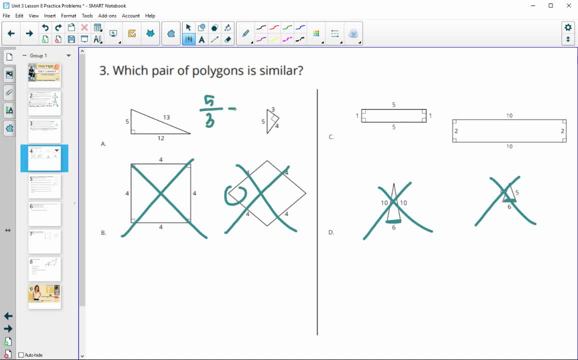 P, S and O into B. Here you're in Lettuce matrix. When V comes in, we find that they are restrict réspec and divide it by the shortest side in the other triangle. so 5 over 3, and then that should be the. 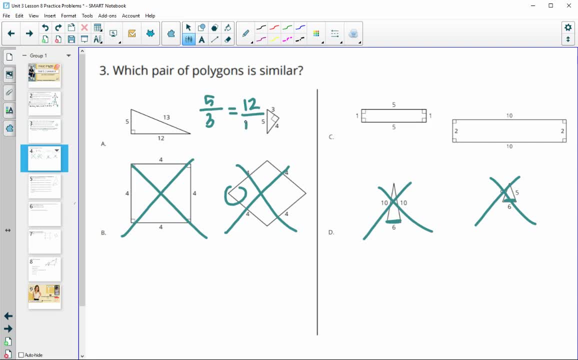 same as if we take the middle side 12 and divide it by the middle side here of 4 and 5 divided by 3 and 12 divided by 4 are not equal, so these sides are not proportional. so a is not good, so we can take a look at c and we see that we have the angles are the same. okay, so the angles. 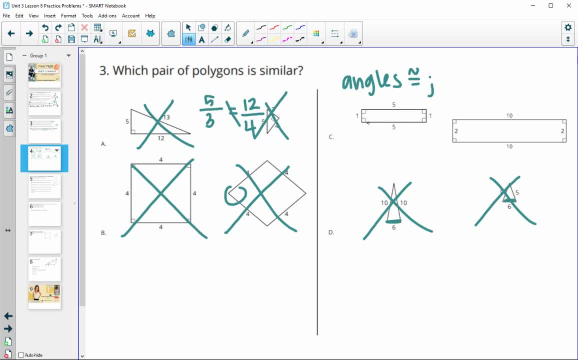 are marked congruent right away. so then we just need to check the side lengths, comparing corresponding sides, so 1 compared to 2, and then 5 compared to 10, and those do simple. both simplify to one half or 0.5, so all of those sides are in proportion. so c has the pair of similar figures. 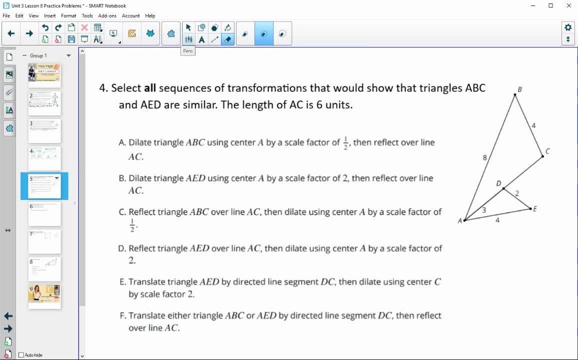 all right. number four wants us to select all transformations that would show that triangle ABC and ADE are similar. And then it also tells us the length of AC is six. So this first one says that we could dilate this larger triangle by a scale factor of a half. 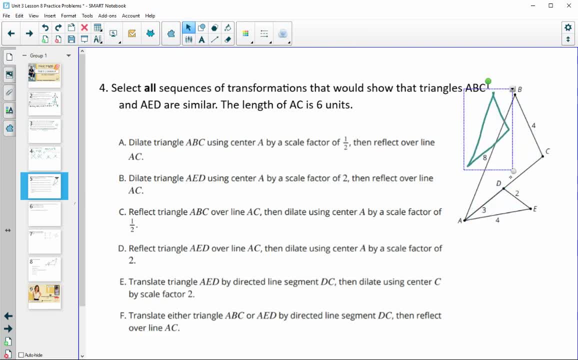 So bring it to half its size. And so if we did that, we know that all the side lengths would match the measurements of AED, since we had eight down to four, four down to two and six down to three. And then it's saying we could reflect it over line AD or, sorry, AC. And then we can see: 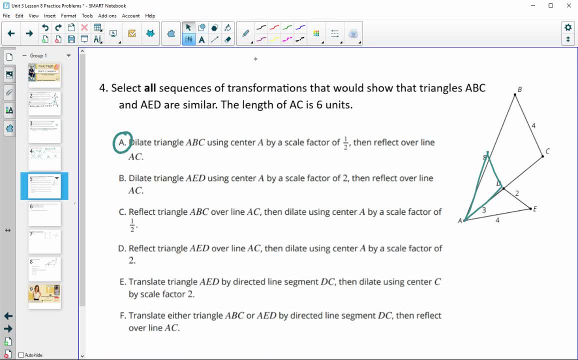 that that would land on this other one, So that would prove similar. B is saying we could, instead of translating the bigger triangle, we could actually translate the smaller triangle, So we could make this one two times the size, So by a scale factor of two, and then flip over. 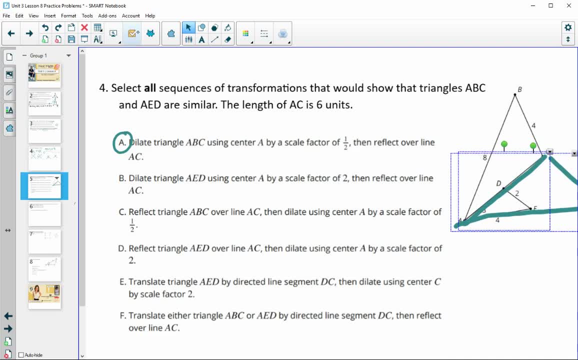 AED And we would see that it would land on that larger triangle. So this B works. C is saying that we could actually do the reflection first, which would be fine, So then we would reflect and then it would be over here, Then do the dilation by one half and bringing it down. So C would work as well. 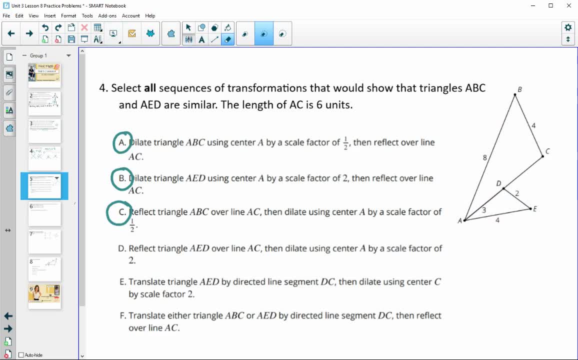 And then a similar idea here, but using the smaller triangle. So D is saying, if we took the smaller triangle and first we dilated it by a factor of two, so doubled its size, and then- or sorry, no, this one's saying- reflect first. 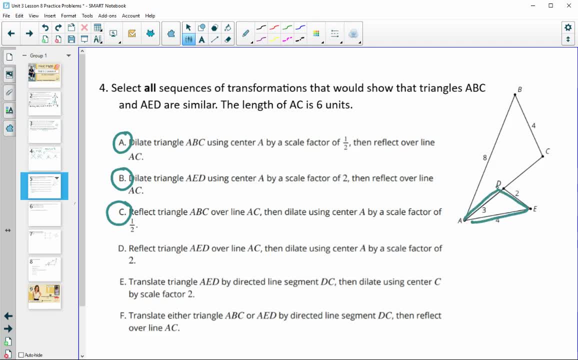 Okay, so take this triangle here and reflect it first, then double the size And so that one would work as well. Final one or final two here work with translations first. So this first one is saying: if we do a translation by segment DC and then we do a dilation by a scale factor of two around C, that that would land it back on itself And that's not going to. we would still need a reflection. So E is wrong. 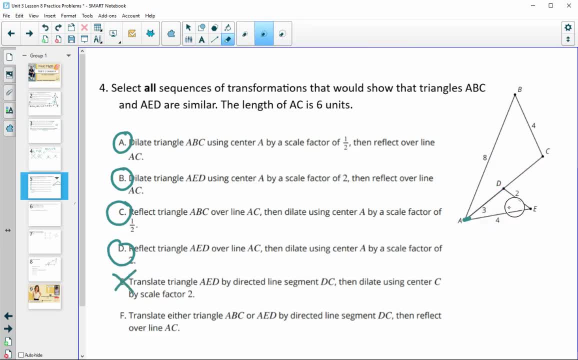 And then F has us do a translation of ABC. And well, it says either. So it says translate either ABC or AED by directed segment DC and then reflect over line AC. So we can see that's not going to land on there either. So F would be false. 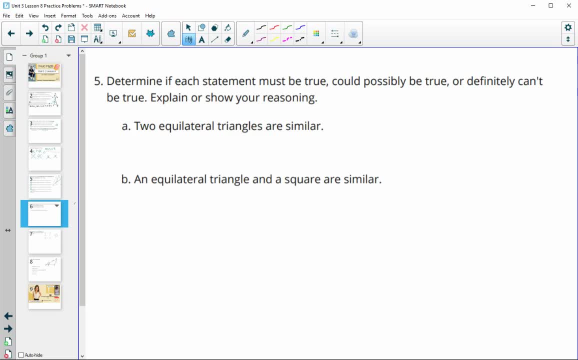 Number five determine if each statement must be true or could possibly be true, or definitely can't be true. So two equal. So the lateral triangles are similar. This one is always going to be true, And that is going to be because the angles are the same. So let me make this a little bit smaller. 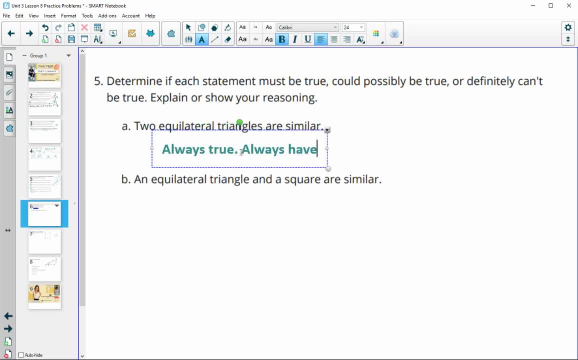 So this is going to be always true because you will always have all 60 degree angles, So we know that the angles will match And we can take a dilation By a scale factor of the new side length divided by the original side length, since all the side lengths are the same, and that's going to put us to the same size triangle. 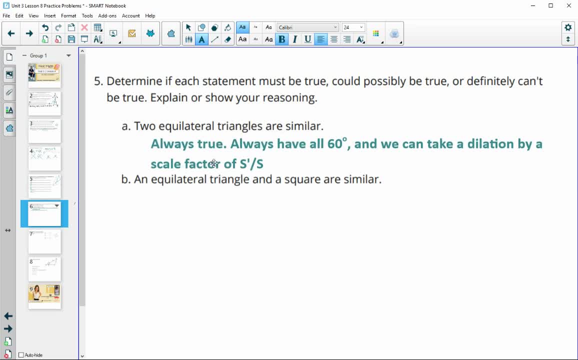 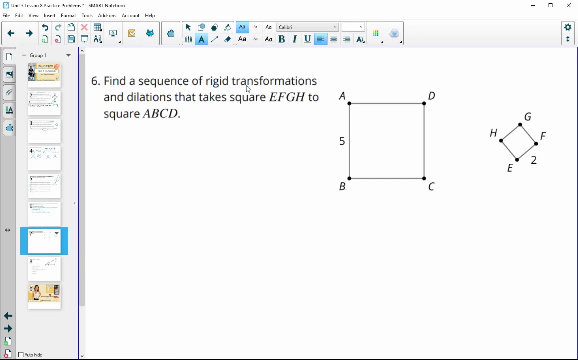 Since all the side lengths were the same, And then this last one. so all equal, or an equilateral triangle and a square are similar. That's going to be never true, Since they aren't the same shape. Okay, Okay, All right. so number six is telling us that we can find a sequence of rigid transformations and dilations that will take E, F, G, H to A, B, C, D. 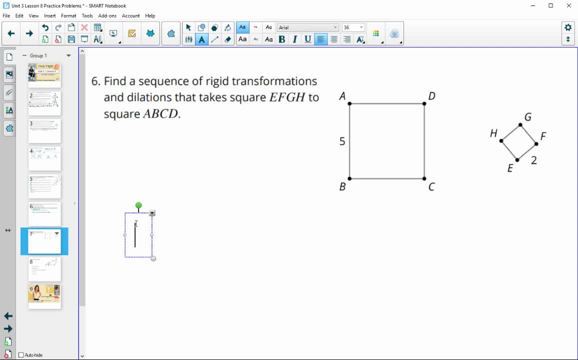 So a couple different ways that you can do this. So I'm going to start with a dilation so that I can get them to the same size. So dilate EFGH to ABCD. So a couple different ways that you can do this. So I'm going to start with a dilation so that I can get them to the same size. 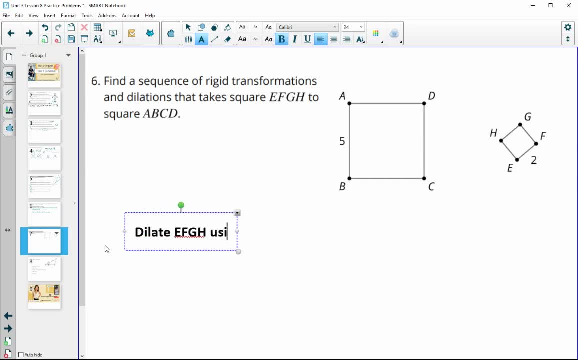 So dilate EFGH to ABCD EFGH, using E as the center and 5 halves as the scale factor. Remember you figure out scale factor by doing the new size divided by the original. So the new is 5 divided by the original is 2.. 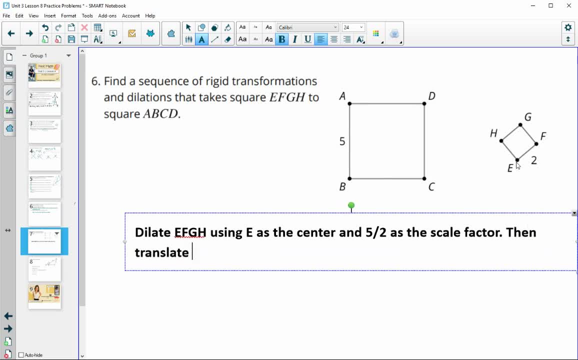 Then I'm going to translate EFGH by directed segment EA, So taking point E onto point A, since they are corresponding. Then rotate EFGH until F coincides with B, So once I get This triangle, Or sorry, this square, to be the same size as ABCD, with that first dilation. 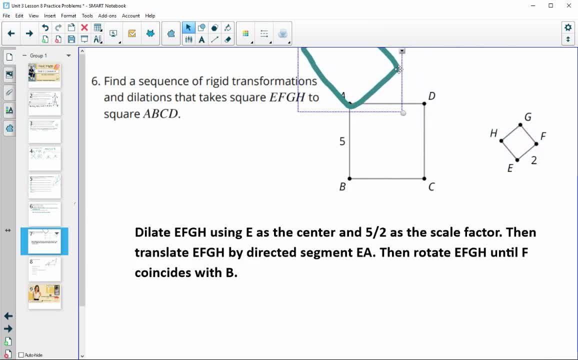 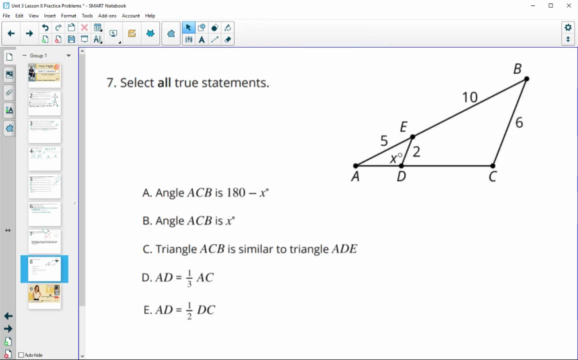 Then I moved E to A and then rotated until this point, Oops, Until this point landed on B, And then that rotated the whole square down to land on top of ABCD. All right number seven. select all true statements. So angle ACB. 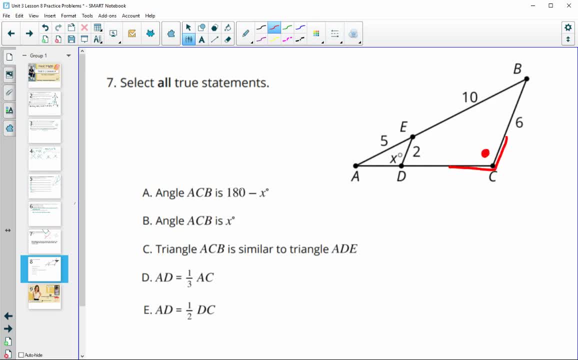 So ACB is this: one is 180 minus X. That would be false, because these two lines are parallel and these are corresponding angles, So they're going to be equal to each other, which is what B says. So they're going to be equal to each other, not equal to 180..